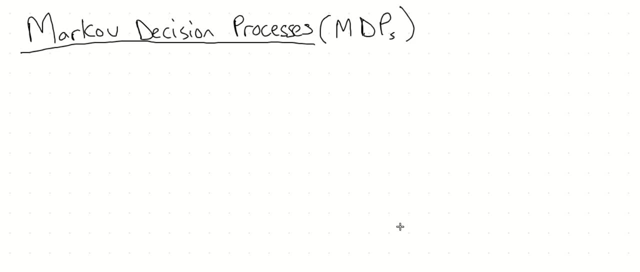 So that means that you know that if you perform this action from that environment in a certain state, it will lead you to another state with this much probability and so forth and so forth. So you understand how the environment dynamics actually work and how any changes. 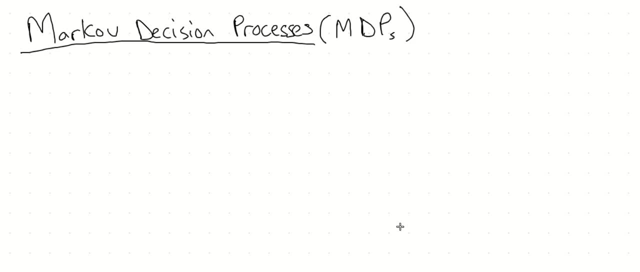 to the environment, or any actions, rather, that you take in this environment, like where would they lead you and with what probability. So if you don't understand what that means right now, that's perfectly fine. That's what we'll be explaining anyway in this lecture and future lectures. 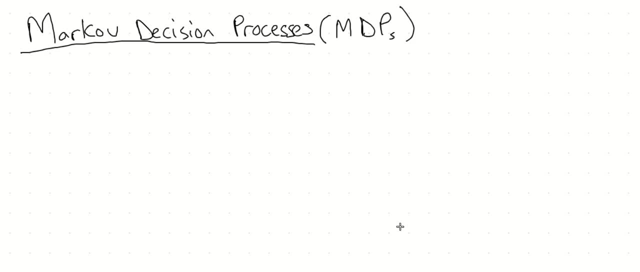 As this is the underlying point behind reinforcement learning problems. So, to start, we're going to go back to our simple diagram that we showed in the previous lecture, where we have an agent And we have the environment. So, like we say that the whole point of reinforcement learning problems are just an interaction between the agent and the environment. it's in 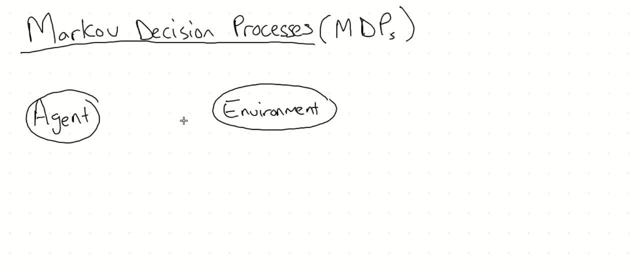 And we showed in the last lecture what examples of what an agent might be, what the environment might be, and so forth, And we'll show more examples as we go on. So what can the agent do? right, The only thing that the agent can do is take an action. 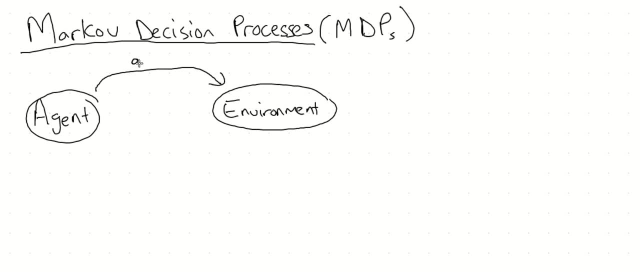 Right. The agent takes an action AT And, based on what action the agent takes, the environment will reward the agent At time step. we'll just say RT plus one. I'll explain what this means. This should be reward And also. 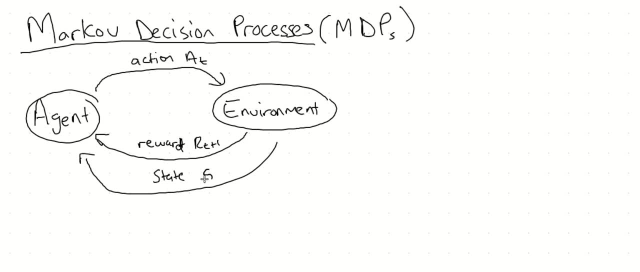 Put the agent in a new state ST plus one, Assuming that the agent started at state ST Right. So the agent started at state ST, He took an action AT And then got rewarded at RT plus one And ended up at a new state ST plus one. 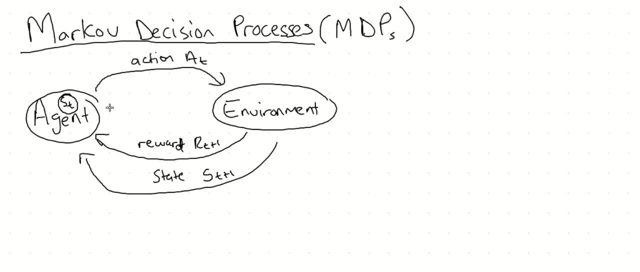 So this interaction kind of continues Like: okay, I'm at some state, I take an action, I get a reward, End up in a new state. I take an action, Get a reward, End up in another state, And it continues until the end of what we call the episode. 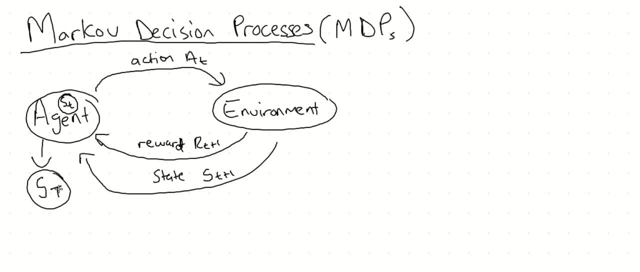 And this happens in time- step Capital T, So ST. This is how we represent what we call the terminal state. Again, it's fine. if this doesn't make sense right now, I'm going to explain what I mean by all this. 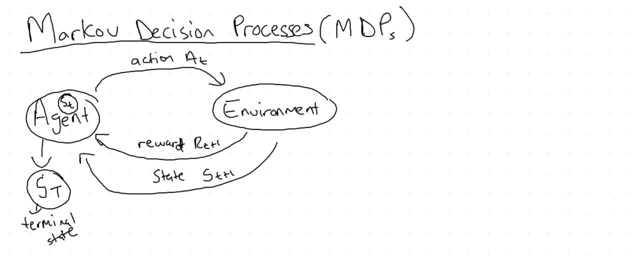 So to actually understand what's happening here, First let's actually draw the timeline Right So we have time: step zero, Time, step one, Time, step two, Time, step three, All the way up to time step N. Okay. 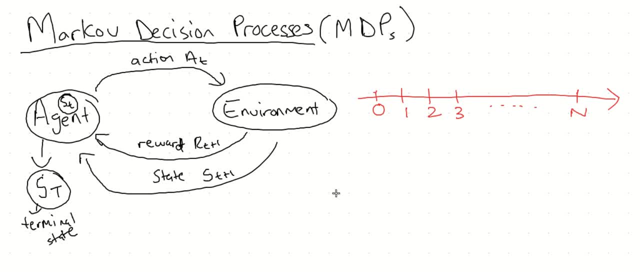 So at each time step the agent needs to make a decision, And at each time step the agent ends up in a new state. So imagine in the following manner: Like at time step zero, you need to make a decision about something. 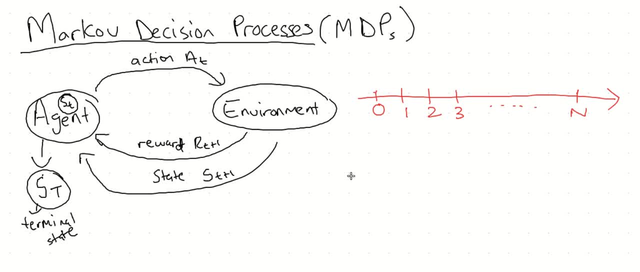 It can be anything, And this decision is what we call an action. So you make your decision Right. Let me use a different color for this. So you need to make a decision Right, Which we'll call A Zero. 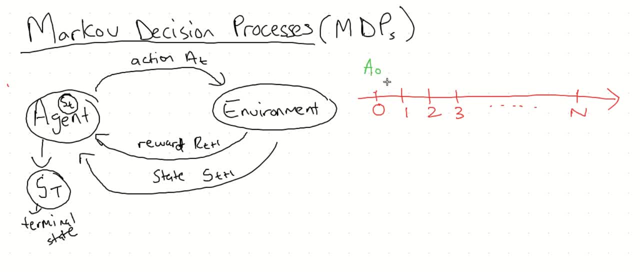 Right, You need to make a decision. After you make a decision, depending on whether it was a good decision or not, you get some reward, which we call R1.. And end up in a new state, which we call S1.. 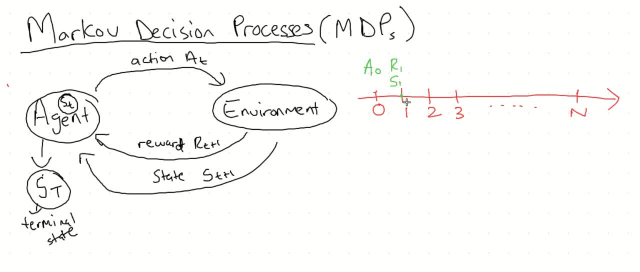 This is at time step one. Now you're at time step one. You need to make another decision, Right? So you make a decision which we call A1. And, based on the decision you make, you get a reward, say R2.. 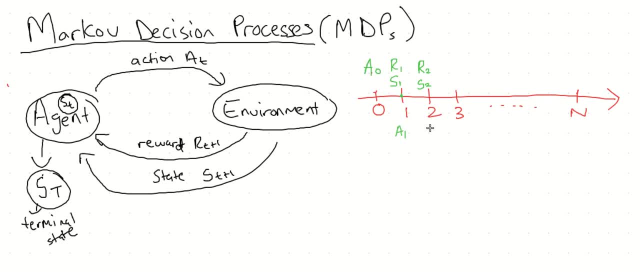 End up in state S2.. And then again, you need to make a decision. You make another decision, which we'll call A2.. You get rewarded- R3.. End up in S3.. You need to make a decision- A3.. 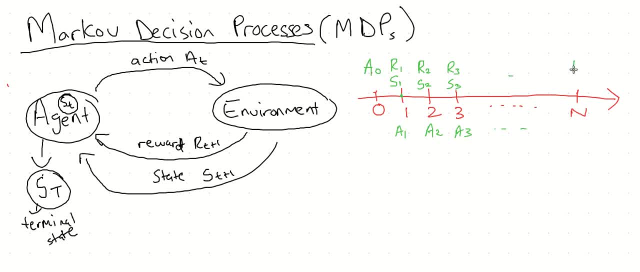 And so forth. Right, Until you get the final reward at time step, which we'll call. This actually was a mistake in my case. Sorry about that. It's actually supposed to be time step T, Capital T, Yeah, Okay. 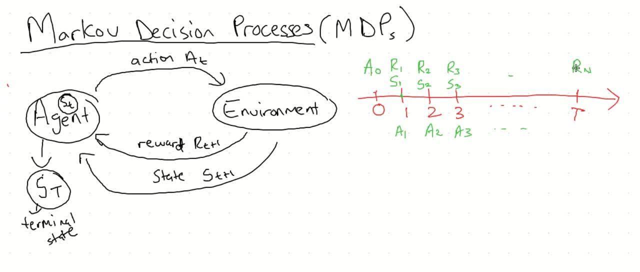 So you get your final reward, R3, here And end up in some final state, S3, which we called the terminal state Right. So again to reiterate what's happening: So you start right In the beginning. 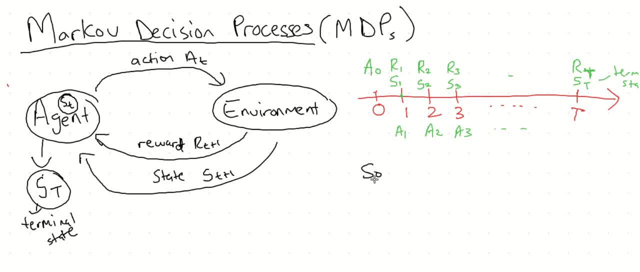 you're in some state S0. You take an action A0. You get rewarded R1.. Now you're in state S1. You need to take an action A1. You get rewarded R2.. 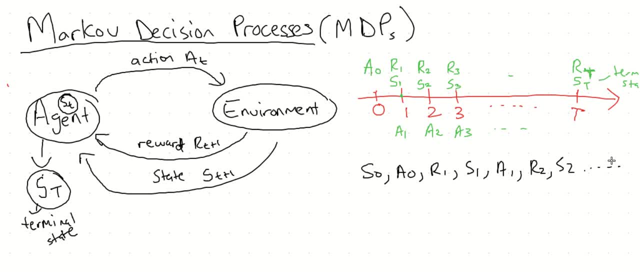 Now you're in state S2. And so forth, And so forth, Until you reach the terminal state ST. This is what we're looking at Like. we are dividing every single thing that we do, every action that we make. 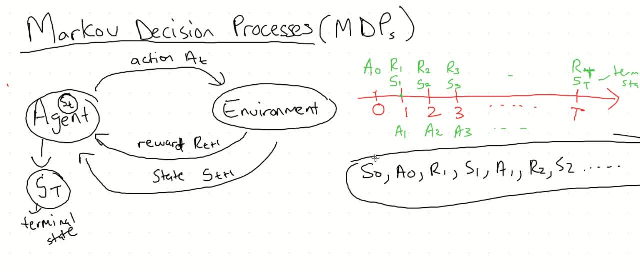 and every time step that we make into this series of actions, This series of time steps and series of actions, reward and state pairs and so forth. So now all of these things are going to happen with some probability. 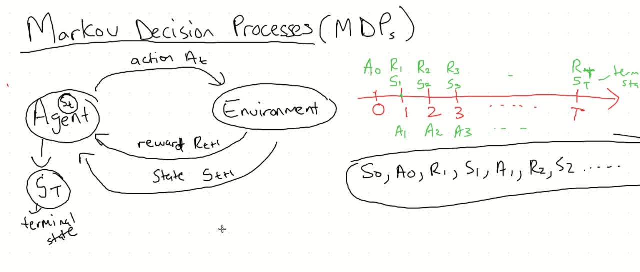 It's not guaranteed that each action will lead you to the same state every time. Sometimes you take an action, it leads you to a state with a certain probability and another state with a certain probability. Right, So let's kind of. 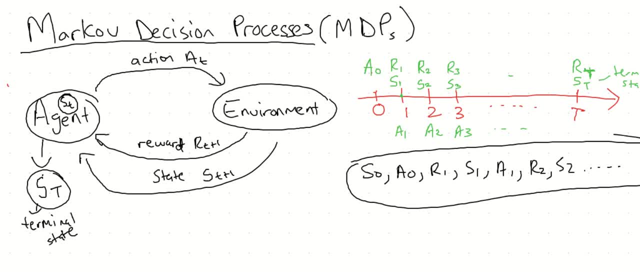 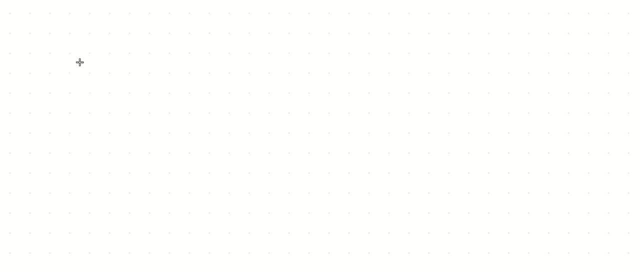 sorry about that. So let's look at what I mean by this. Imagine you start in a state S0.. If you remember, from here, we defined S0 as our initial starting point. right, This is where everything starts. 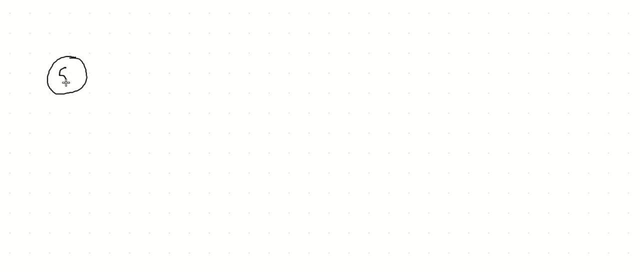 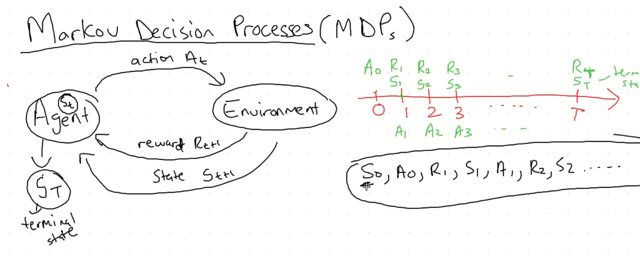 and then everything starts again. So S1, S2, S3,, S4,, S5,, S6, S7, S8, S9,, S10,, S11, S12,, S13,, S14,. S15, S16,, S17,, S18,, S19,, S20,, S21,, S22,, S23,, S24,, S25,, S26,, S27,, S28,, S29,, S30,, S31,. 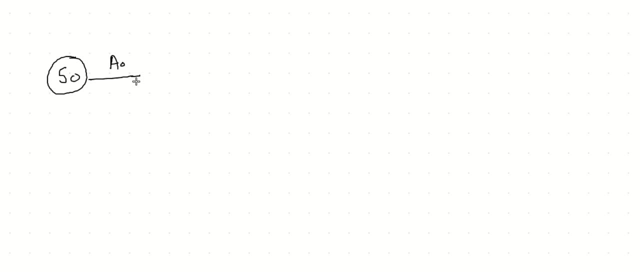 S32, S33, S34,, S35, S36, S37, S38,, S39,, S40,, S41, S42, S43, S45,, S46, S47,, S49,, S50,. S51, S52,, S53,, S54, S55, S56, S57, S58, S59,, S60, S61, S62,, S63, S64, S65, S67, S68,. S69,, S70,, S71, S72,, S71, S72,, S73,, S71, S72,, S73,, S71, S72,, S71, S74,, S74,, S7,, S7,. 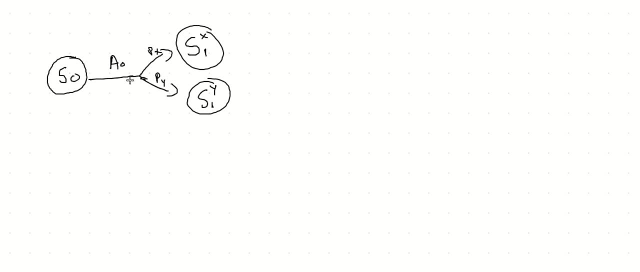 S8, S8, S9, S10, S11, S11, S12, S13, S14, S15, S16, S17, S17, S19, S19, S20, that we need to know for the environment and why markov decision processes are actually kind of 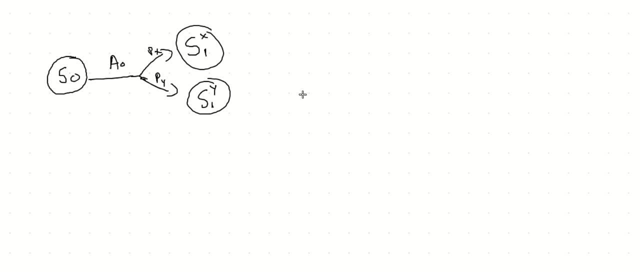 important to understand here. so i'll go on to say that if someone asks you like, okay, you need to take an action. but before you take an action, uh, as a rational person, you need to think like: oh, what's the probability that this action is going to lead me in the state that i want to be in? 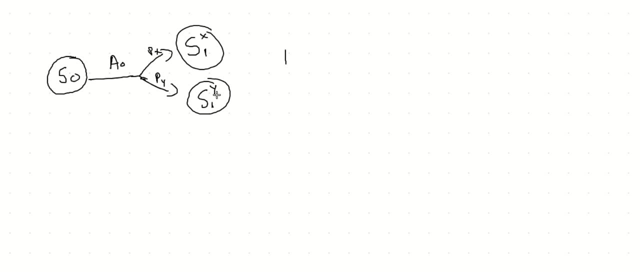 maybe you want to be in s1x, but maybe s1y is so bad that you don't want to be in it. so if px is really high and the probability of you being in s1x the state that you actually want to be in. 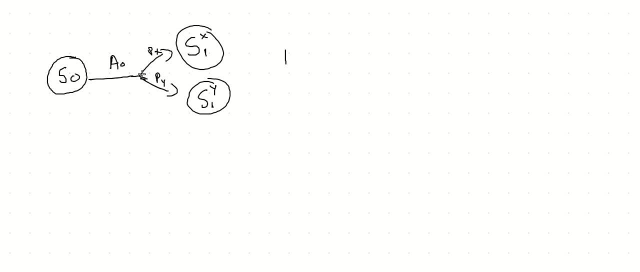 uh, is actually high, then maybe okay, a0, it should be the action you take. otherwise, maybe it's better to take another action right, and we'll go into this later on. but so an important thing to actually know is what's the probability of me ending up in the state that i actually want to be in? 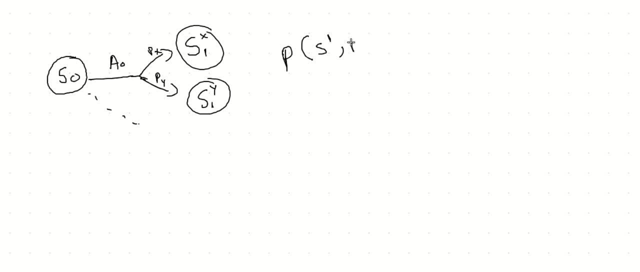 some state, which called s prime getting some reward r, given that i'm in some state s and they take action a. so, given that i'm in s0 and i take a0, what's the probability that i end up in s1x or s1y? that's what s prime here is, so this probability is quite important and is actually known as a. 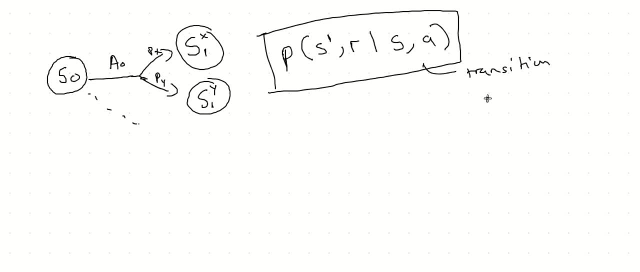 transition probability, and this is essentially the model for our environment, right? uh, this is, this is our model. so if we know, uh, what this uh big um set of probabilities are for a whole environment, and if then we can actually start solving, uh developing algorithms to solve for this mdp and so forth, right, one important thing to note here is: 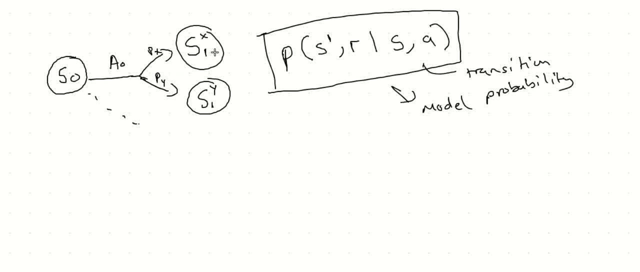 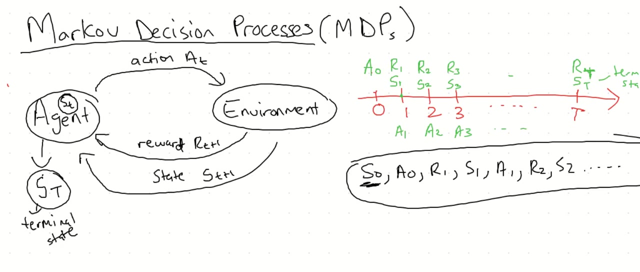 that we are just when we're trying to estimate s1, x, s1y or s prime. so we're trying to estimate this, this uh, probability right of being in s prime. we are only concerned with the state s right. but if you look at here, if we go back here, 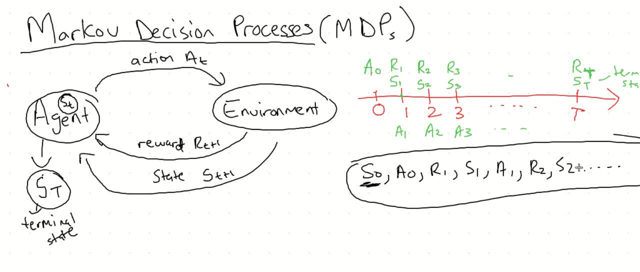 and someone asked you that- what is the probability of generally ending up in state s2? right, this probability depends on what happened before: r2, a1, s1. it depends on all those random variables, but we are only concerned with uh, the very last one, which means the very last uh state we're in. 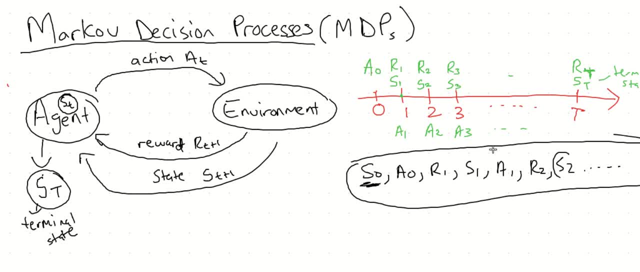 should be able to summarize all of the information that has happened in the previous state. this is called the markovian assumption, right hence the name markov decision processes. you can, of course, look more into what this means, but, um, basically, uh it what we're disregarding, or say we're just assuming that. 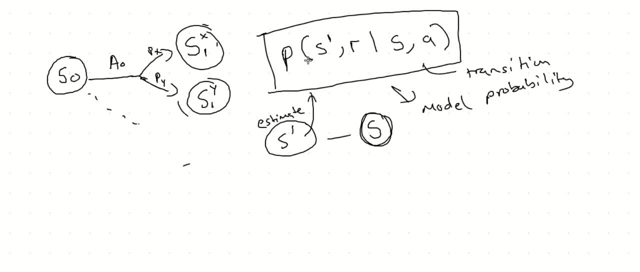 the probability, uh the probability of ending up in s prime or ending up in state? uh, let's say s t plus 1. this probability will depend on what happened in the previous state. s t only, and anything else before that we don't care about it. so st minus one, s t minus two. 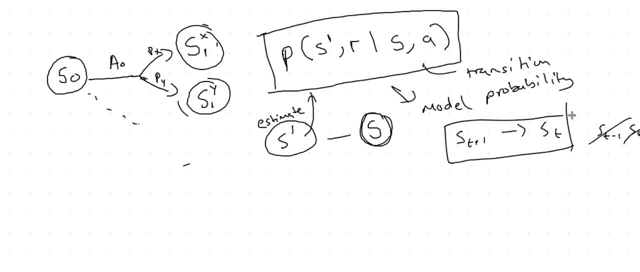 right, we disregard all this. we just look at this kind of evolving formulation like from s, t plus1 one. we just concern ourselves with ST and this is a very huge assumption to make, but we'll soon realize that it's important for us to make use this. 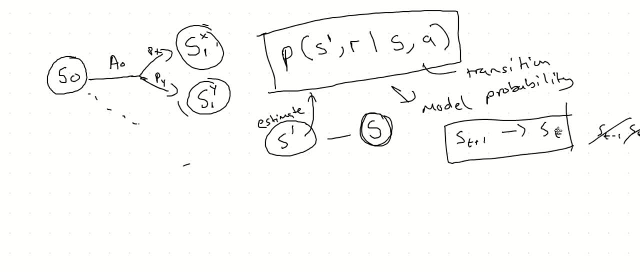 assumption, so that we for solving the problems that we're gonna be solving- and I'll go into detail again in future videos of what that means, so it's not to confuse you early on in the lectures, right? so this is actually quite important to know. and another property, and this will be the focus of the next: 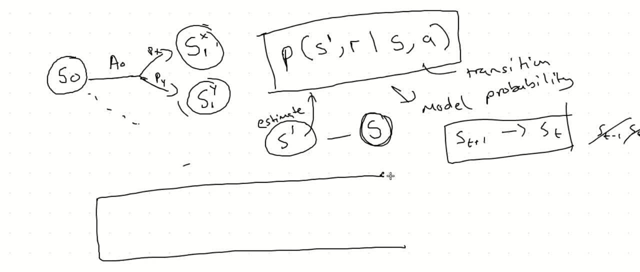 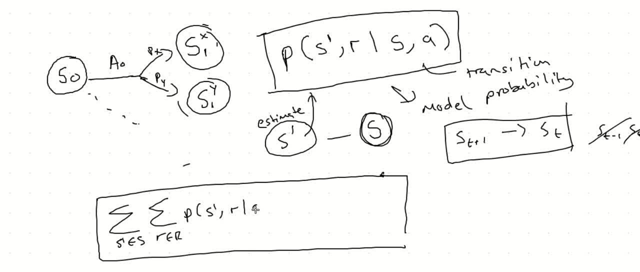 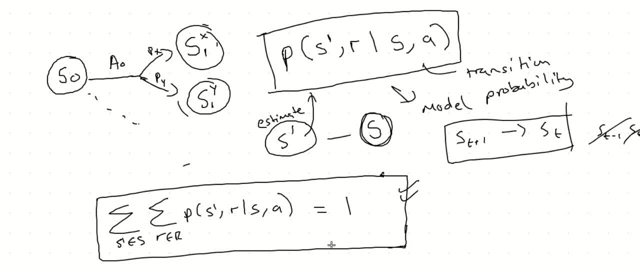 is to convince yourself why this is the case, right given what I just explained before and, of course- like I'm gonna go into detail in the next video of how- why we're actually saying this is the case with it all came from, but for now I'm 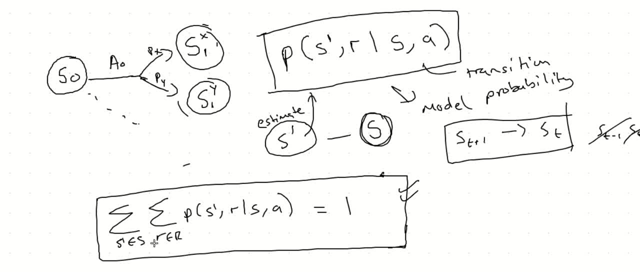 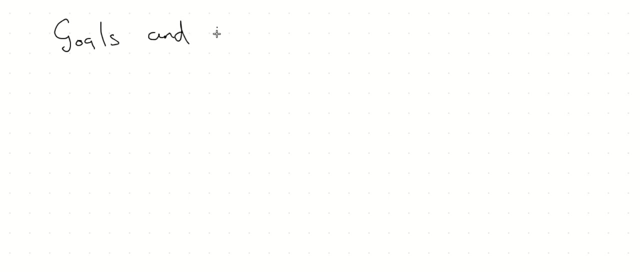 just gonna leave it as is at this point and we will move on to the next step, which is focusing on goals and rewards. like we what we are actually trying to solve for when we're solving for reinforcement learning problems. so look at goals and rewards so we know that the reward function is kind of like the 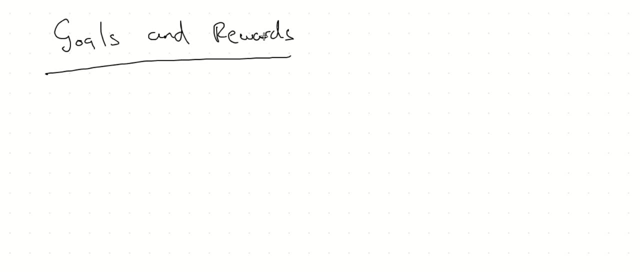 most important thing is what signifies our learning process when solving, for reinforcement learning problems. right, and this reward function is, of course, just represented by RT, a simple numeric number that's just saying that, okay, your reward for performing this action is positive, this or negative of that, right? so it's just some scalar. uh, of course, if you look at in the magnified view, 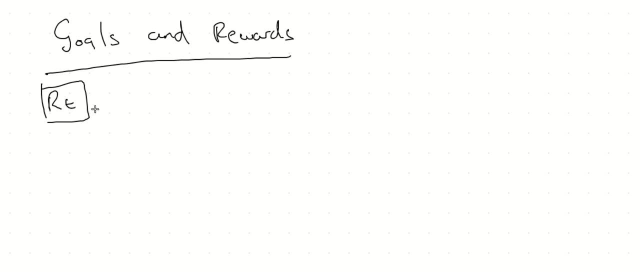 then of course it can be a matrix and so forth, but that's not the point of this. and we say that we divided, if you remember, earlier we divided all our episodes, as we'd call them, all our events right into time, steps right, all the way up to some time, step t right. so this is how we 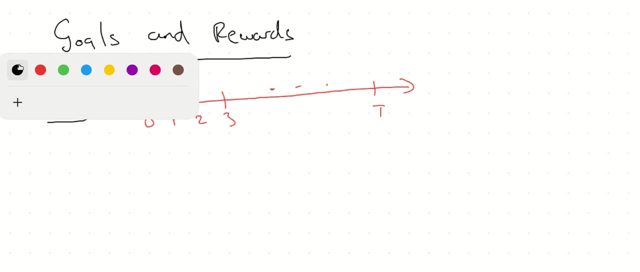 divided everything. now, based on this, we should be able to determine what our goal is right. we, if you remember, for the first lecture, don't care about short-term rewards. so we don't care about what happens at time- step one. but we care about what happens at time- step one. 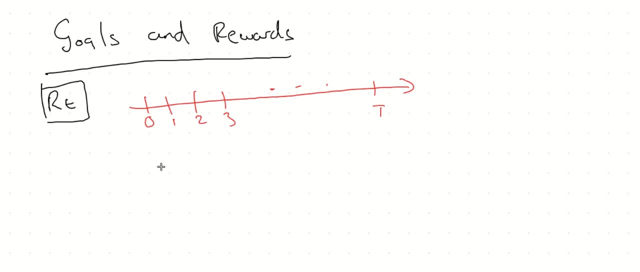 we don't care about what happens at time step one, we don't care about the sum of all rewards until time step t. so what we are trying to actually maximize is not our rewards, but rather the accumulation of rewards known as the return right. this is what we want to maximize, and the return is represented by 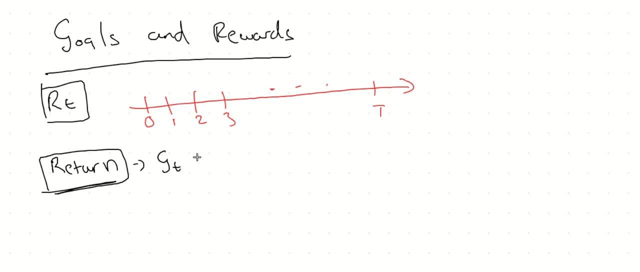 gt right. so gt is equal to the summation of all rewards: rt plus one plus rt plus two plus rt plus three, all the way up to rt capital t right. and this is happening at the final time step. so now that we know that, okay, what we want to maximize is the return. this happens in episodic cases, like when we can define a return. 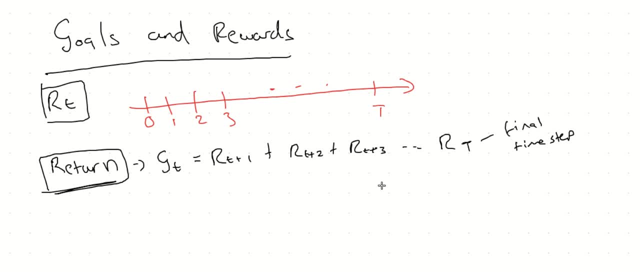 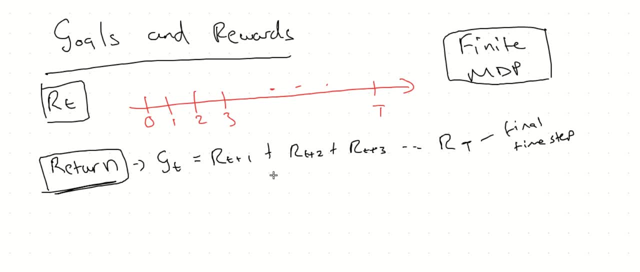 maybe it's an infinite episode or something like this. so that leads us to a dilemma whereby we might just continue getting towards more and more and more in the future and our episodes never actually terminate. so that leads me to a question for you. if someone offered you ten thousand dollars, 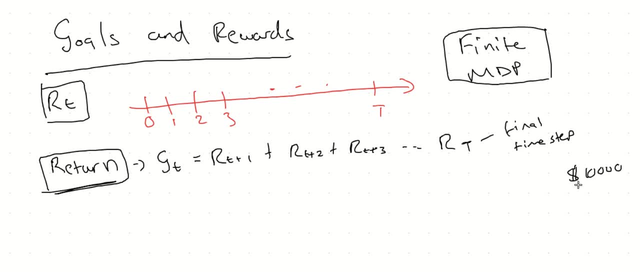 today and ten thousand dollars, let's say, uh, in two years time, right, which one would be more valuable to you? right and based, most people would probably answer that having it today is more valuable because having it in two years there's a whole uncertainty element that comes down with. 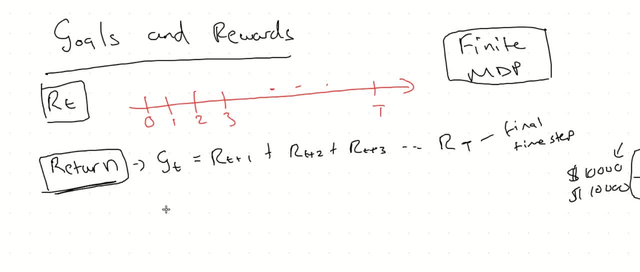 it, and the same goes for reinforcement learning problems. the rewards that we're gaining now are actually more valuable than the rewards that we'll get in future time steps, because in future time steps the uncertainty grows right. so essentially, what we need is to discount the future rewards right, and what we do like uh for discounting. 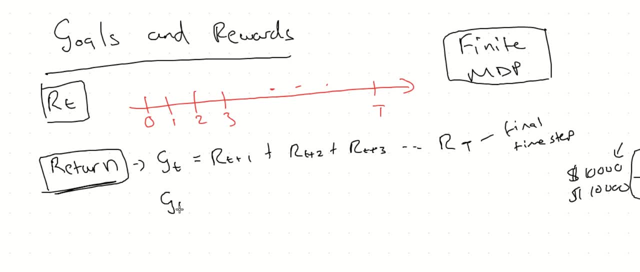 those rewards is essentially redefining our gt to be equal to rt plus one plus gamma. rt plus two plus gamma. squared rt plus three. right, all the way right up to gamma. this would be rt. right, this would be gamma rt minus one. sorry so, gamma rt minus one, with a variety. so 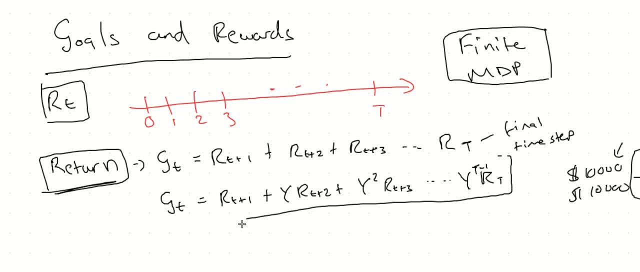 this becomes our return right, and the important thing to know is that gamma should be actually between zero and one right. this is also an important property for gamma, so gamma is just a discount factor that actually shows that we care about immediate rewards more than we do about future rewards, and it's also important to discount our rewards in the case of. 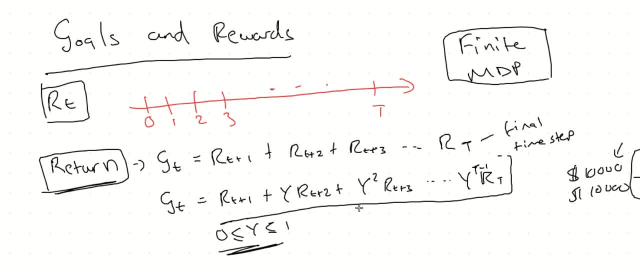 infinite mdps, because when we have infinite mdps, then like, uh, the if we don't discount our rewards, then, uh, we'll never terminate our algorithms and you'll see why in future videos and when we go through our programming lectures, like why we're saying that this will never terminate. 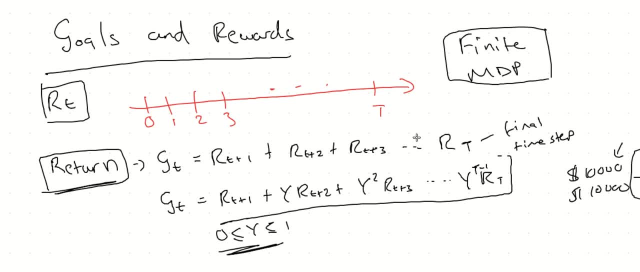 and you just try to convince yourself: uh, why, that is for now, but we'll go through it again in the future. so essentially what we are doing is uh, for each uh time step that we gain a reward, we discount it and so forth, for two reasons. one is to deal for the